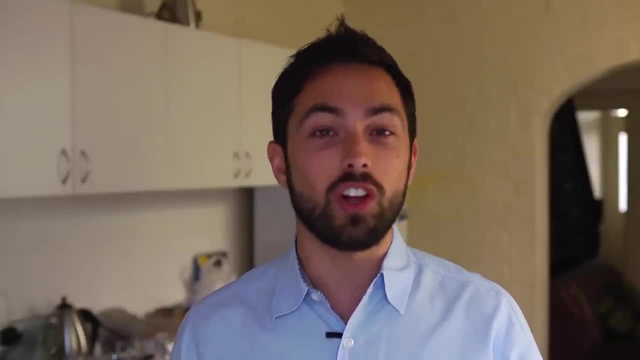 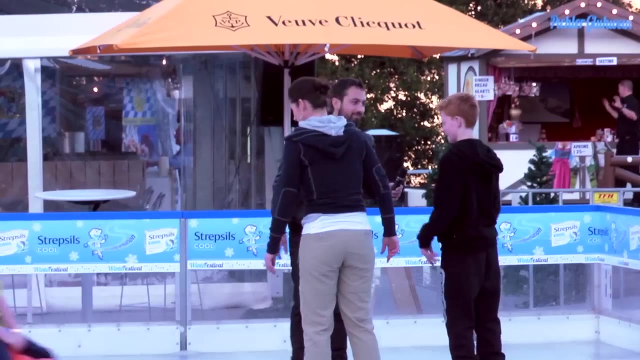 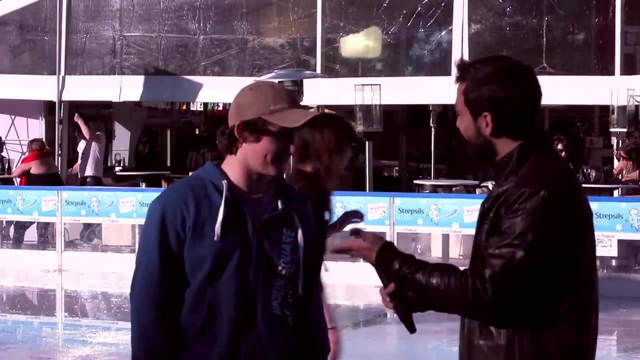 I guess we got there in the end. So what's the difference between solid and liquid water? So obviously the temperature of it. It's a lot colder. Ice is frozen. What does it mean to be frozen then? Cold, Cold Liquid water is no good for skating on. Ice is great. 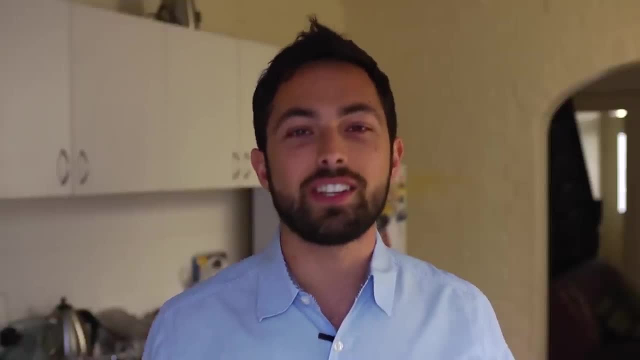 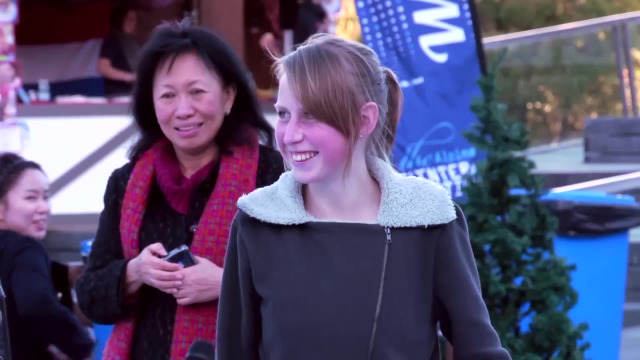 Nothing other than temperature. So everyone recognizes that temperature is important in determining whether the water is ice or liquid. But what's actually happening between the water molecules? What's the difference between water and ice? It's frozen. What does it mean for something to be frozen? 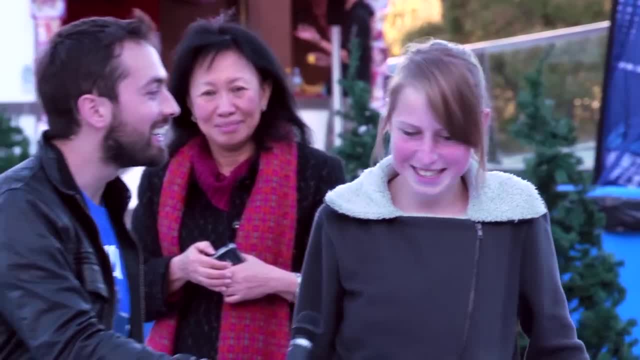 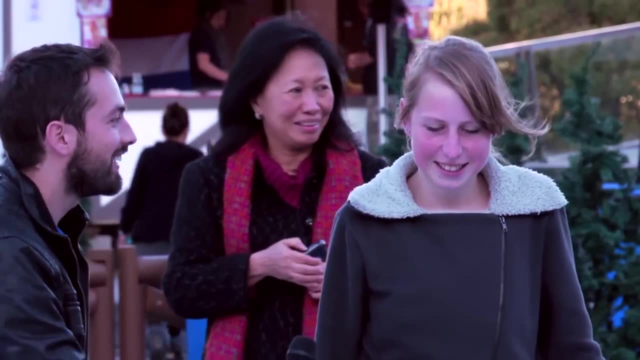 It's solid. What does it mean for something to be solid, That it's like a brick? It's like a brick. It's like a brick. And what makes it like a brick? What's happening in there? I don't know. 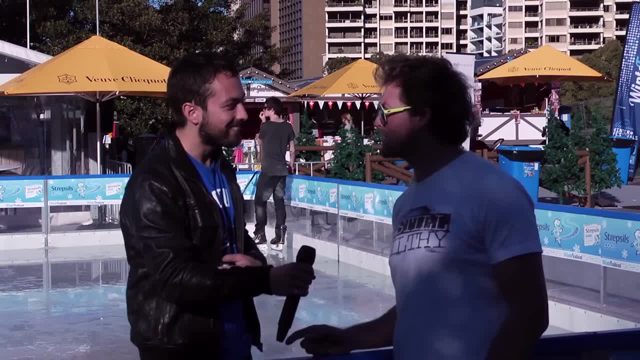 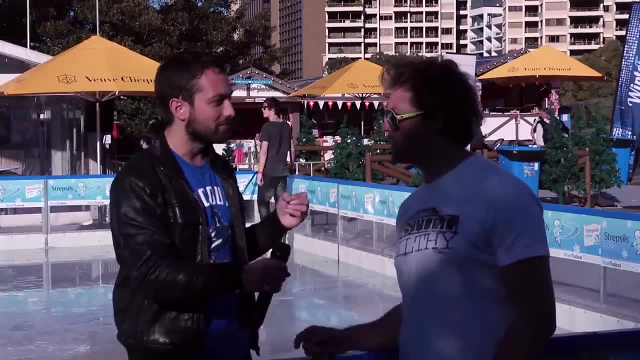 But what makes it a solid versus a liquid? Well, in this case, lots of pipes going underneath. That makes it very cold. Makes it very, very cold. yeah, But what's actually happening to the little bits of water They're attaching to each other? 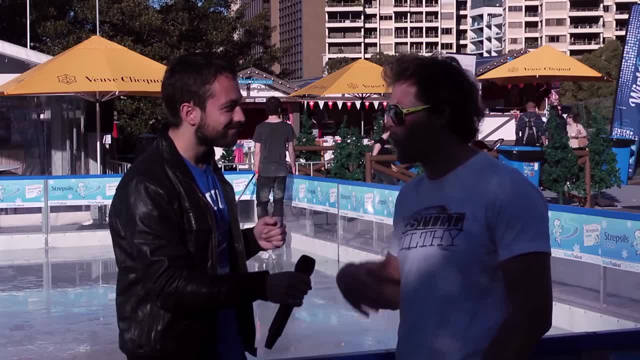 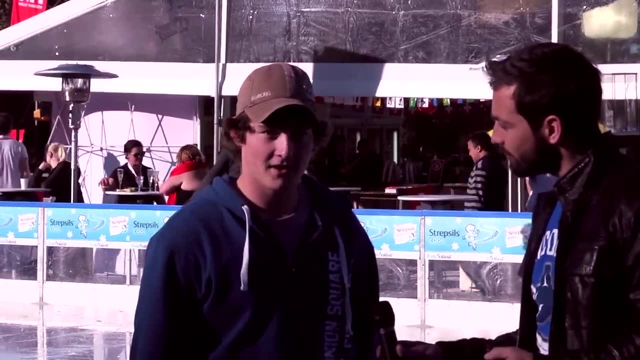 This is all the guesswork here. I imagine they're attaching to each other, They're forming a more solid end to piece. You cool liquid water down and then at some point, what happens to it? It slows down, freezes and stalls. 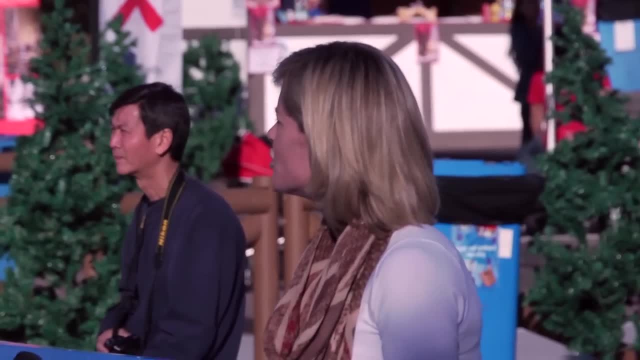 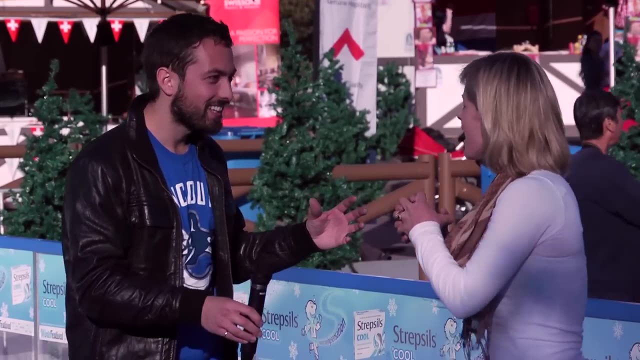 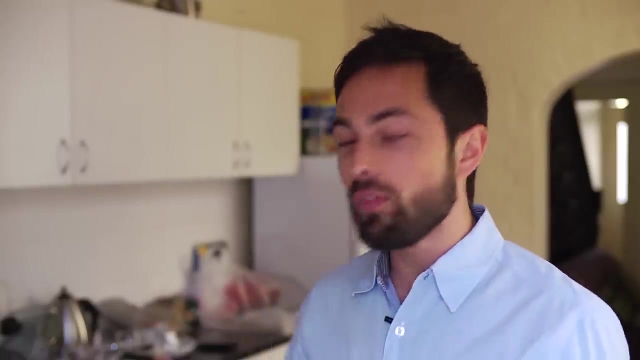 Freezes and stops moving, The molecules become frozen. How do they become frozen? They join together, They accumulate, They coagulate. Coagulate is not the technical term for it, but everyone was on the right track. In ice, the water molecules are basically fixed in place. 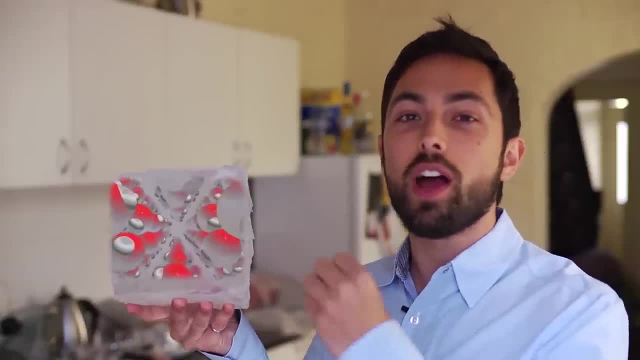 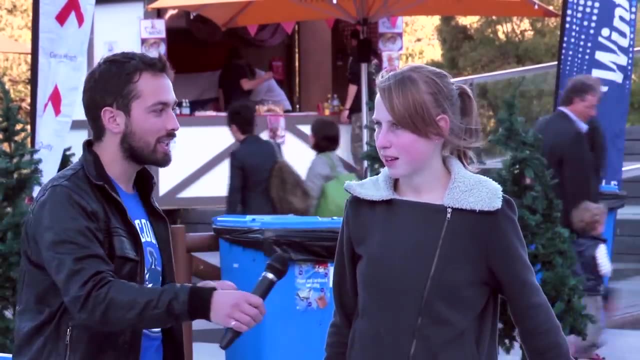 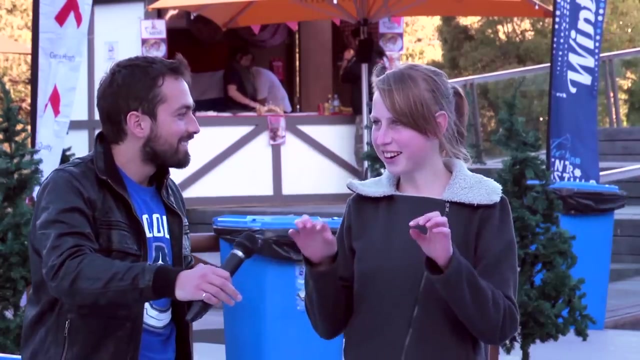 They form a crystal lattice where their only motion is vibrating. So what happens if we heat up the ice? What happens when a solid melts? They all bounce out and melt. What are we talking about? What are they doing? In science, you draw little circles. 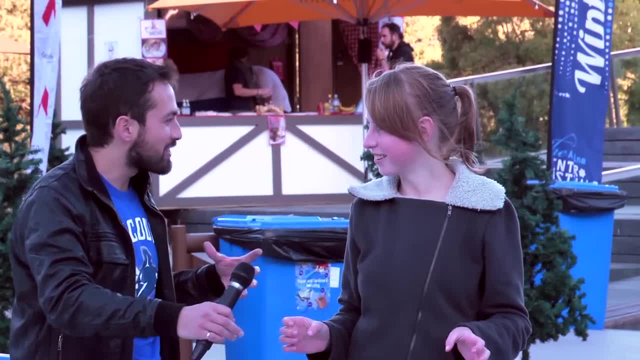 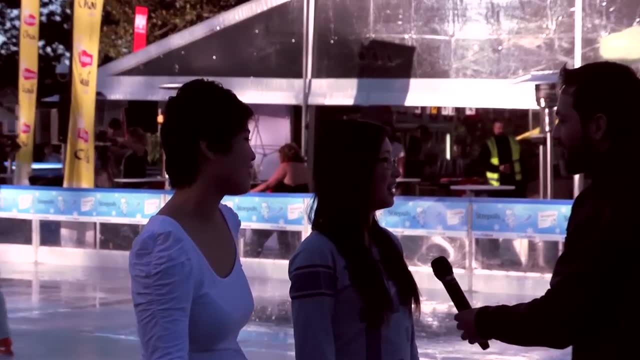 What are those little circles? Oxygen, Are they just oxygen, Hydrogen oxygen, And the two And the two. The temperature is higher. So the particles: they're less stable, Less stable, Not stable. They're more free to move around. 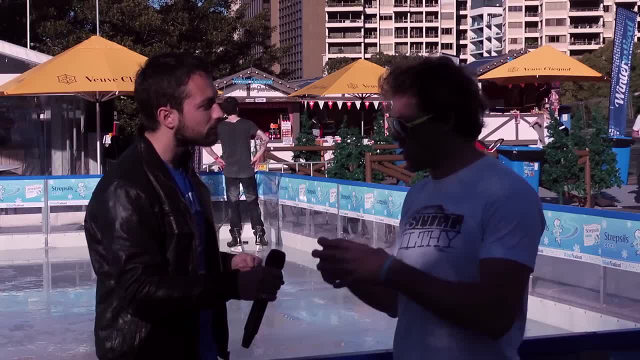 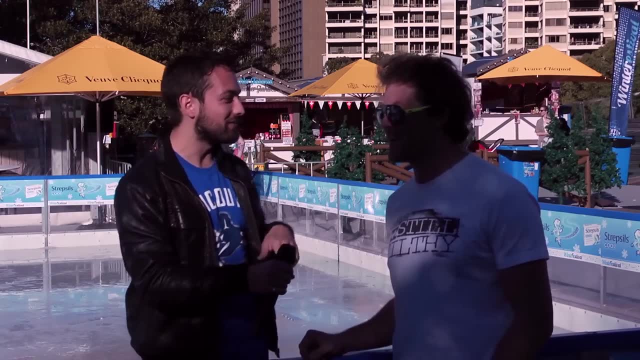 That sounds right. They become separate and they are allowed to move around, And in gas maybe they're further apart. Is that what we're? This is fantastic. This guy has nailed it Alright. that makes sense now. That's awesome.